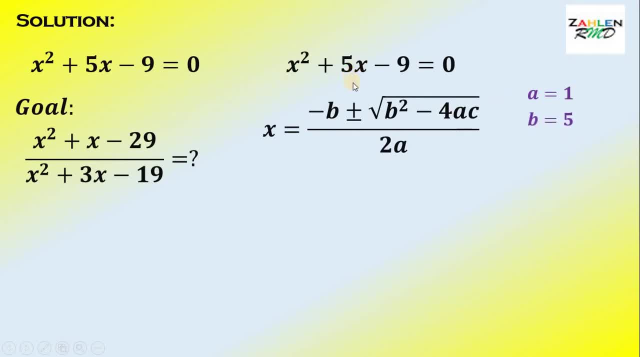 And the value of b is the coefficient of x, which is 5.. And the value of c is the constant term of this equation, which is negative, 9.. Substitute all the given values and we have x equals negative, 5.. Plus or minus square root of 5, squared minus 4 times 1 times negative, 9 all over 2 times 1.. 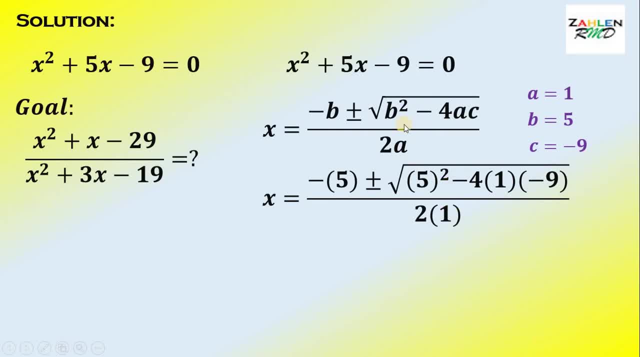 Now, at this point, a becomes 1,, b becomes 5, and c becomes negative 9.. Now simplify and we get: x equals negative, 5 plus or minus square root of 61, all over 2.. Now this is the value of x. 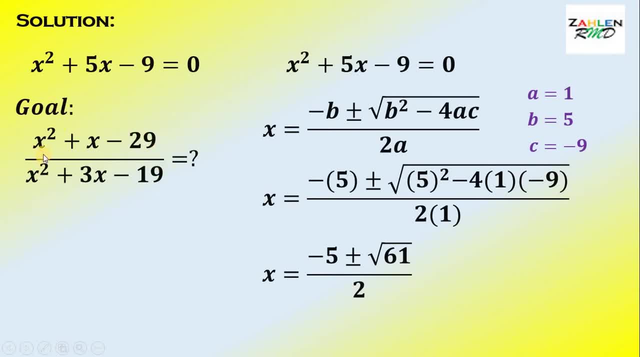 Now, if you want to find the value of x, you need to find the value of x squared plus or minus square root of 5 squared minus 4 times 1 times negative 9 all over 2 times 1.. Now, if you want to find the value of x squared plus x minus 29, all over x squared plus 3x minus 19,. 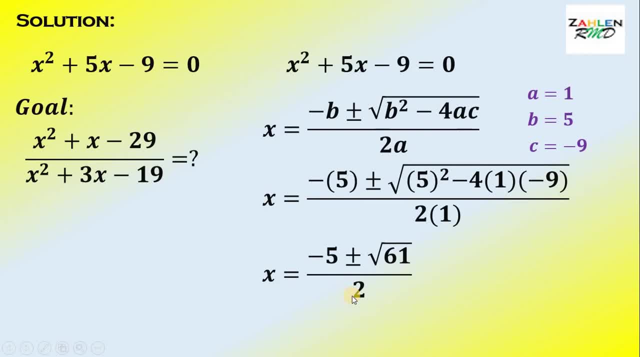 we need to substitute the value of x, And this equation gets messy. That's why the instruction is: without solving the equation. Now the question is what we're going to do to find the value of this expression without solving this equation. Now, first thing to do is to focus on the equation. 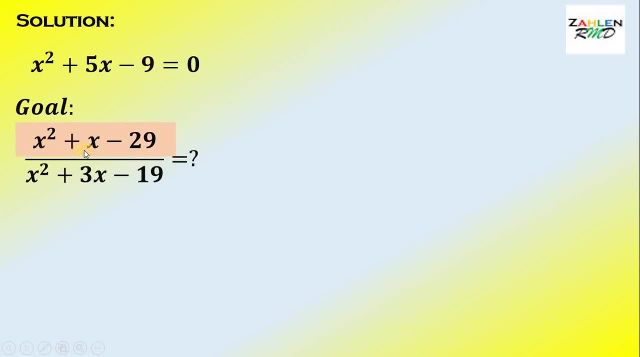 So what we're going to do is to focus on this numerator. We have x squared plus x minus 29.. And what we're going to do is to rewrite this equation Now. x can be written as 5x minus 4x, and 29 can be written as 20 plus 9.. 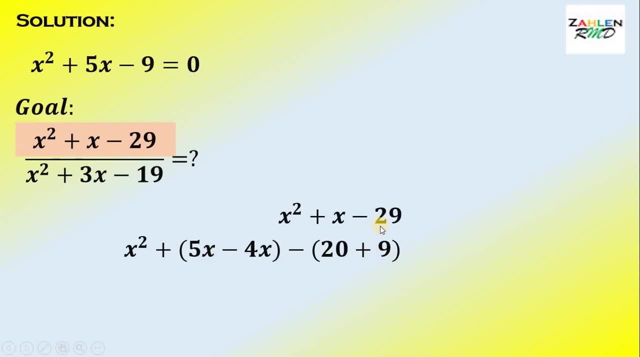 So again, x is simply 5x minus 4x and 29 is 20 plus 9.. Now distribute the negative sign. We get x squared plus 5x minus 4x, Minus 20 minus 9.. 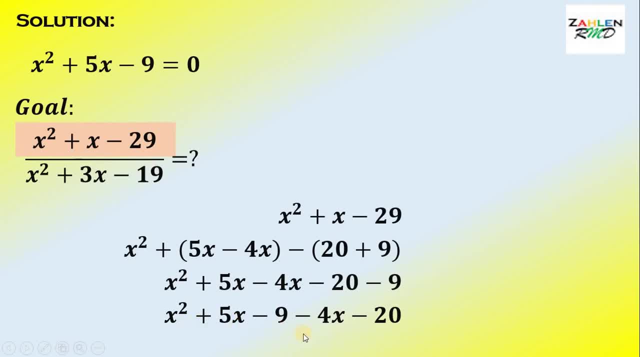 Now rearrange. We get x squared plus 5x minus 9, minus 4x minus 20.. Now don't forget that x squared plus 5x minus 9 is equal to 0.. Therefore, this x squared plus 5x minus 9 is gone, or simply 0..